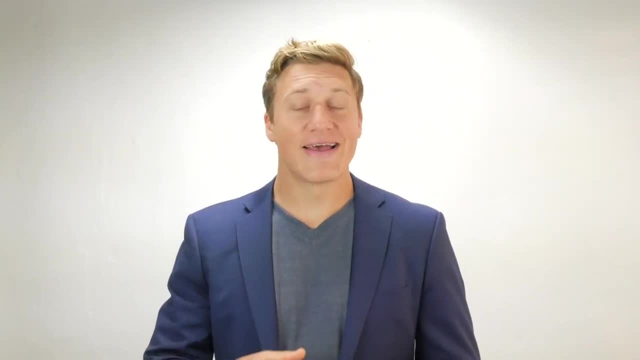 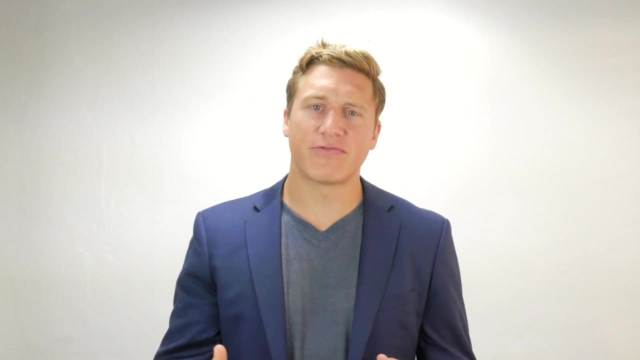 Filing your taxes can be a headache if you aren't familiar with the process. Thankfully, all of the information you need for your W-2 is located directly on your pay stub. This information can give you an idea of approximately how much your tax return will be. 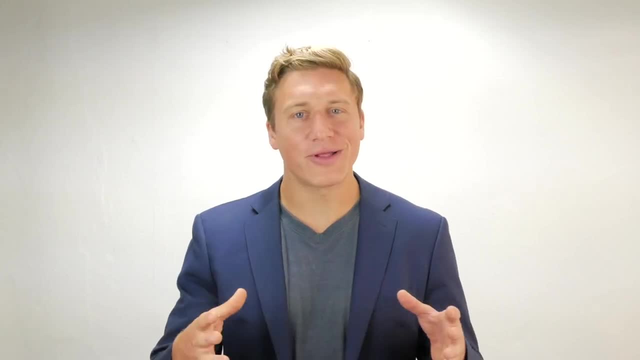 The pay stubs have created this guide to help you learn how to calculate your W-2 wages- Taxable Income. To start to calculate your W-2 wages, you'll want to look at the year-to-date totals on your most recent paycheck For the most accurate. 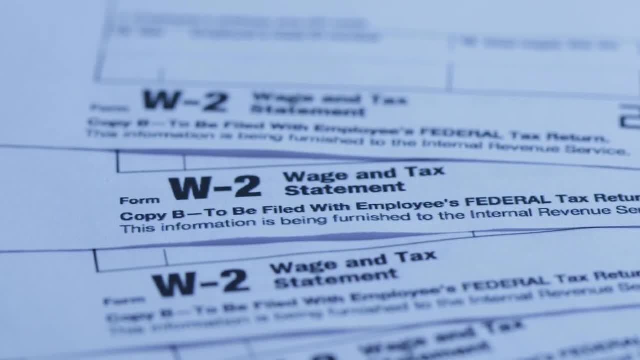 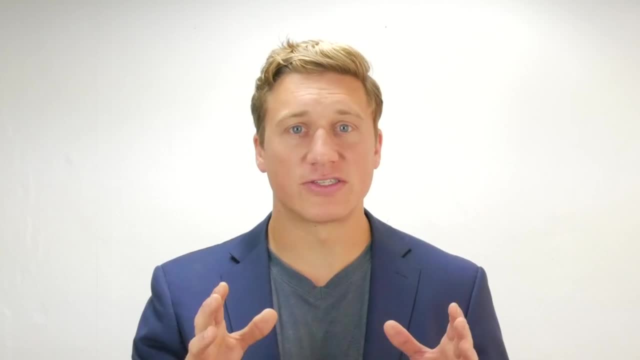 results. you'll want to get this information from the last paycheck of the year. This will have the total of all the wages you've earned that year. This amount may need to be adjusted if you have any deductions that are excluded from taxable income. These deductions include: 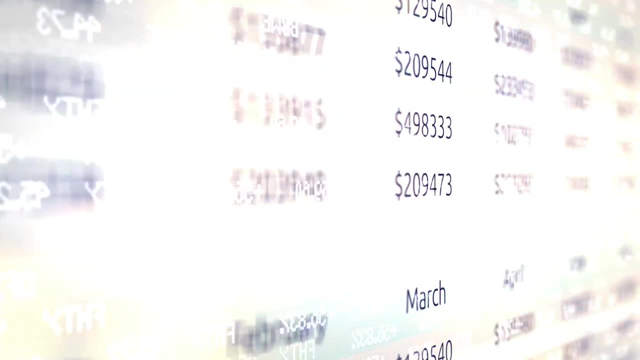 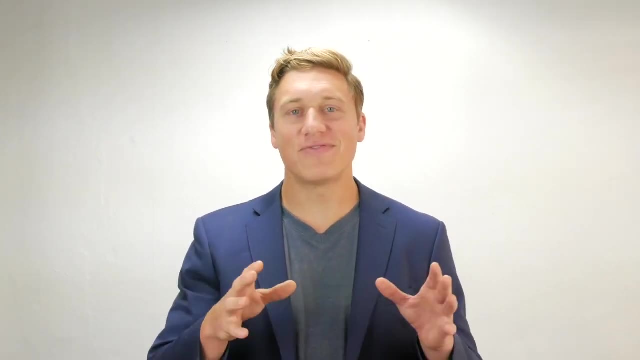 401 deductions: premiums for health insurance, premiums for group of life insurance, vision and dental insurance premiums, and dependent care reimbursement accounts. You'll subtract any of these items from your gross taxable wages. The number you get should match the number you see. 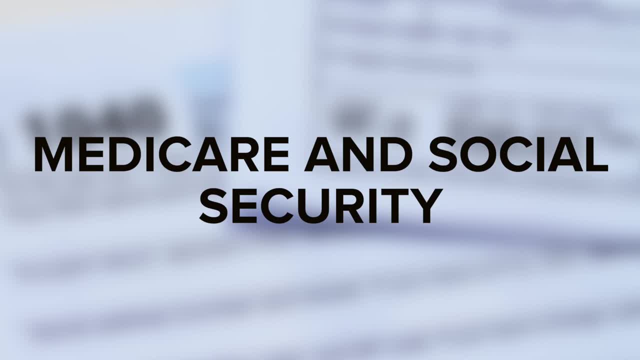 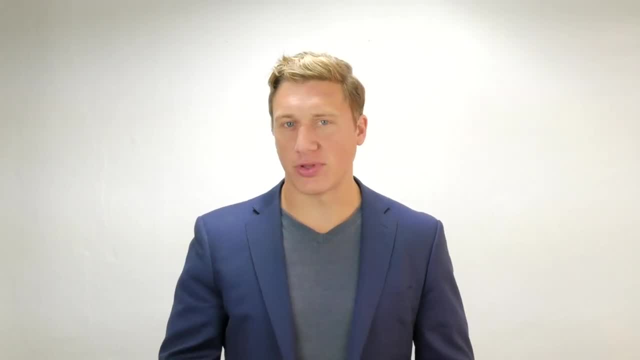 in box 1 on your W-2. The number you get should match the number you see in box 1 on your W-2.. Calculating your W-2 wages for Medicare and Social Security taxable wages is similar to finding your taxable income. The difference is there's a maximum amount of wages that 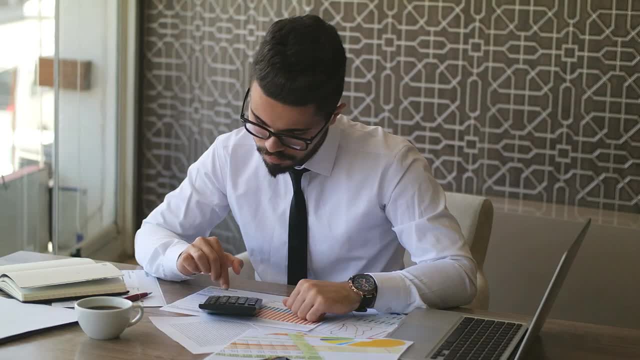 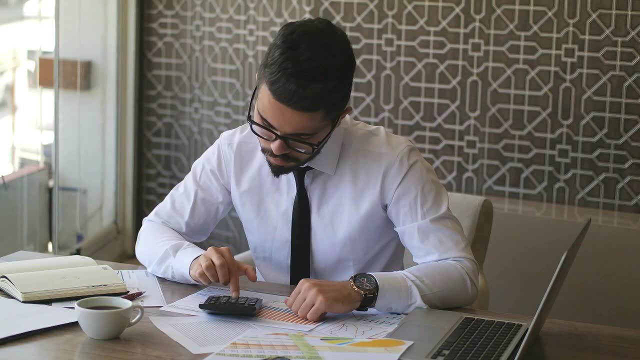 is taxable for Social Security tax. Again, you'll start by looking at your most recent pay stub. Look at the gross taxable income for the year to date. You'll take this number and subtract any pre-tax deductions. These will be similar to your federal and state wages, but not identical. 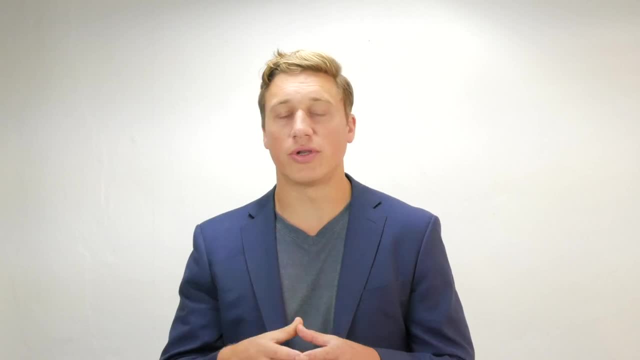 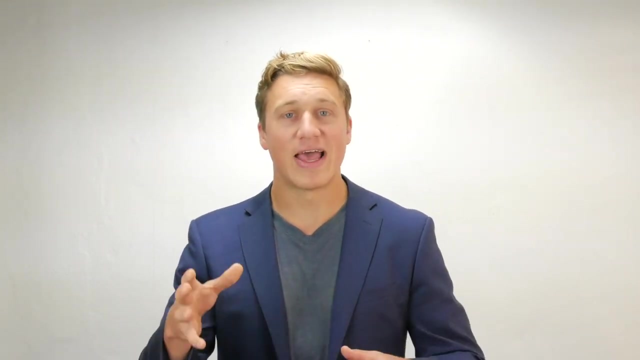 Pre-tax deductions for Medicare and Social Security include insurance premiums and life insurance premiums. You'll also want to deduct any employer paid benefits you may have received throughout the year. Each tax return situation is unique. Your personal tax return will depend on your personal exemptions and expenses throughout the year. It's also important 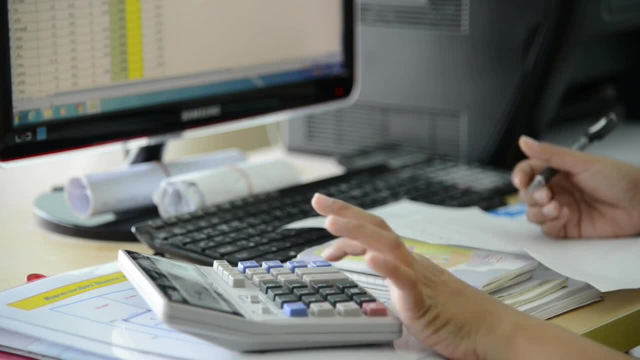 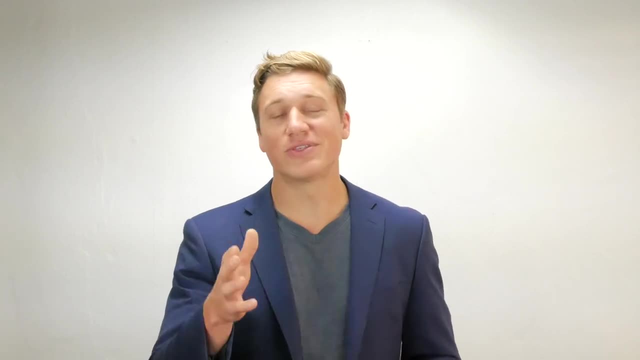 to note that using your pay stub to calculate W-2 wages is just an estimate. You may have additional personal exemptions that should be included. You could either do these manually or use the pay stub's W-2 form generator to create your document automatically in minutes. 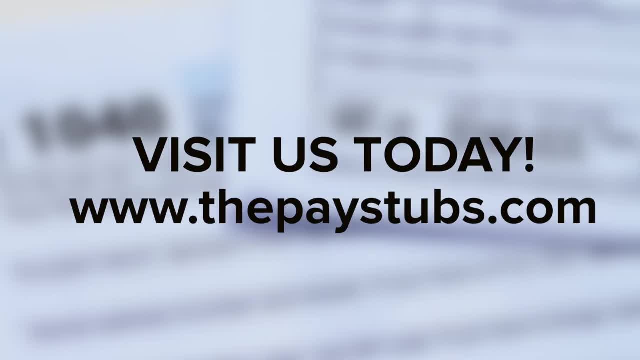 Visit us today to calculate your taxes and generate a form W-2.. If you liked this video, be sure to like, comment and subscribe.